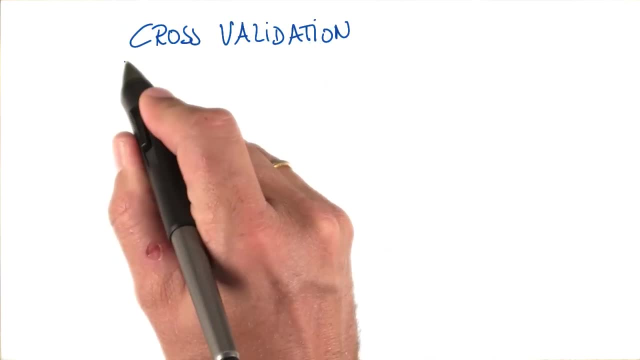 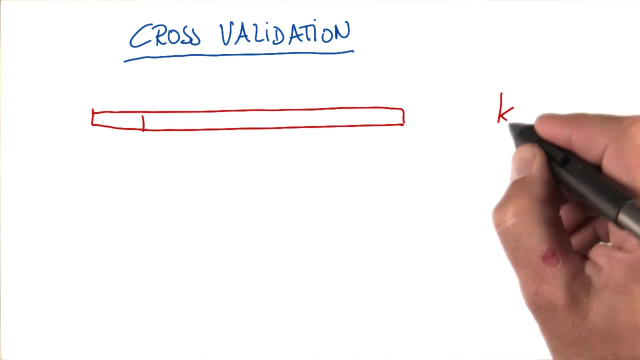 is lost for the training set. So where do we set this trade-off? And this is where cross-validation came into the picture. The basic idea is that you partition your data set into K bins of equal size. So, example: if you have 200 data points and 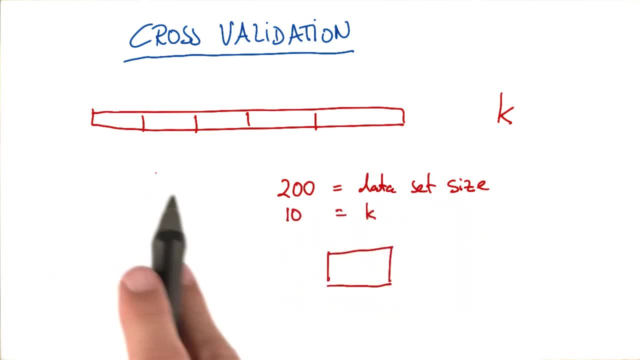 you have 10 bins very quickly. what's the number of data points per bin? Quite obviously, it's 20.. So you would have 20 data points in each of the 10 bins. So here's the picture, Whereas in the work that Katie showed you, 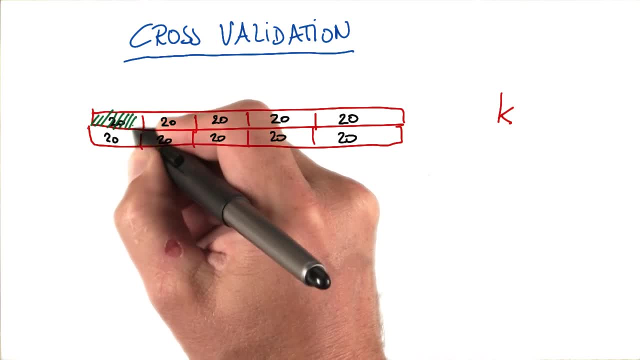 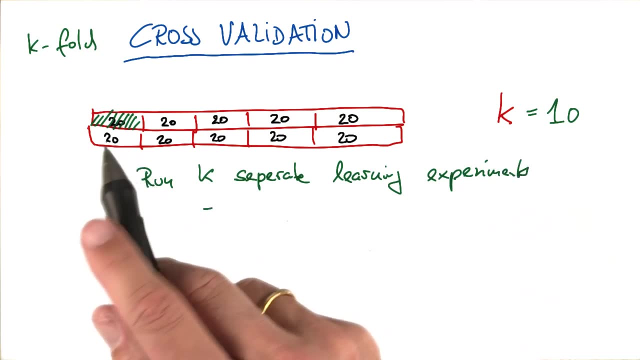 you just pick one of those bins as a testing bin and the other one as a training bin. In K-fold cross-validation you run K separate learning experiments In each of those. you pick one of those K subsets as your testing set. The remaining K-1 bins are put together into 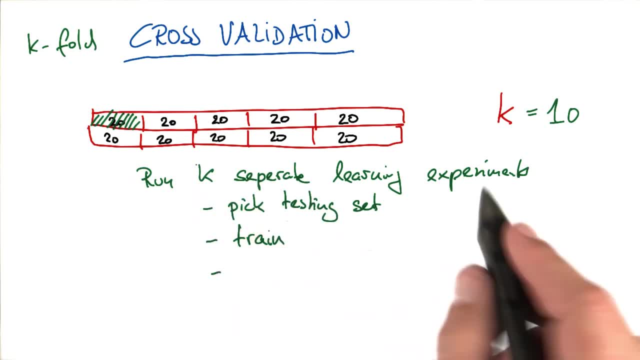 the training set. Then you train your machine learning algorithm and, just like before, you test the performance on the testing set. The key thing in cross-validation is you run this multiple times- in this case 10 times- and then you average the 10 different testing set performances for. 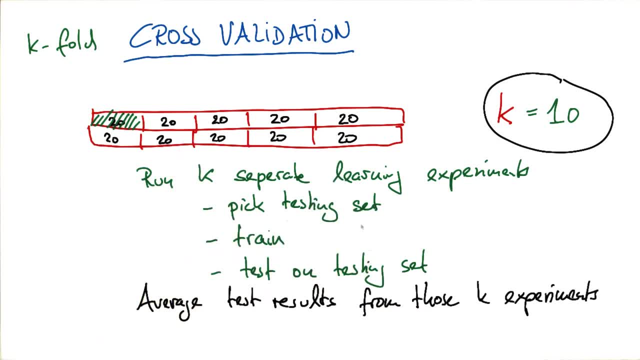 the 10 different holdout sets So you average the test results from those K experiments. So obviously this takes more compute time because you now have to run K separate learning experiments. But the assessment of the learning algorithm will be more accurate And in a way you've kind of used all your data for training and 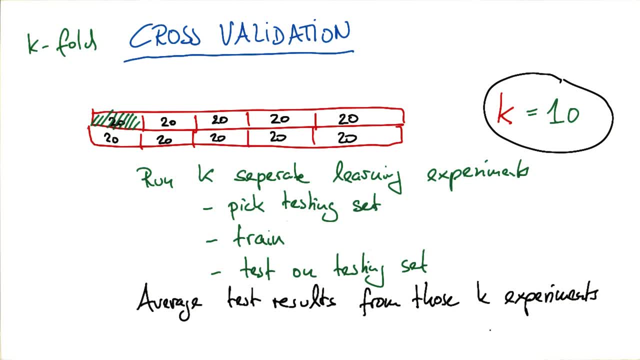 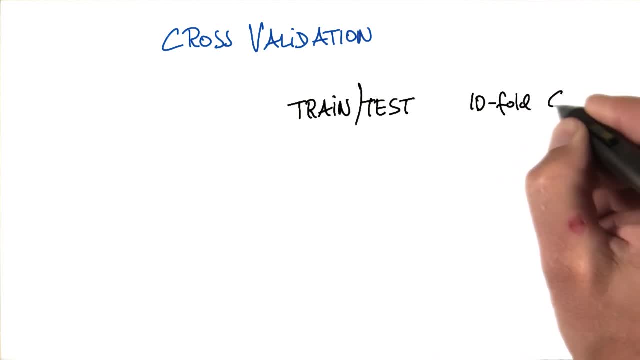 all your data for testing, which is kind of cool. Let me just ask one question. Suppose you have a choice to do the static train test methodology that Katie told you about, or you do, say 10-fold cross-validation CV, And you really care about minimizing training time, minimize run time after. 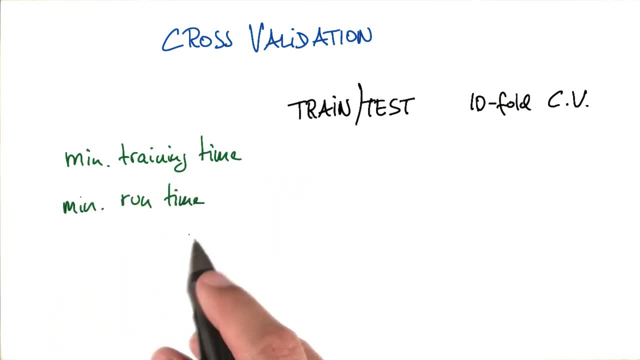 training using your machine learning algorithm to output past the training time And maximize accuracy. In each of these three situations, you might pick either train test or 10-fold cross-validation. Give me a best guess. which one would you pick? So, for each minimum training time, pick one of the two over here on the right. side.